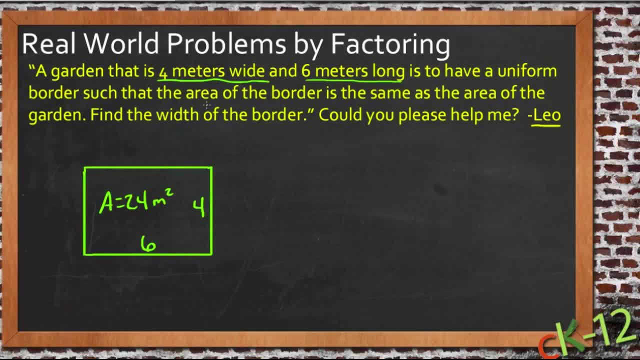 Then he says it has to have a uniform border. so a uniform border means that the border is going to be the same width all the way around. So when we're done the garden is going to be. obviously the overall plot will be bigger than it is now. and if that border 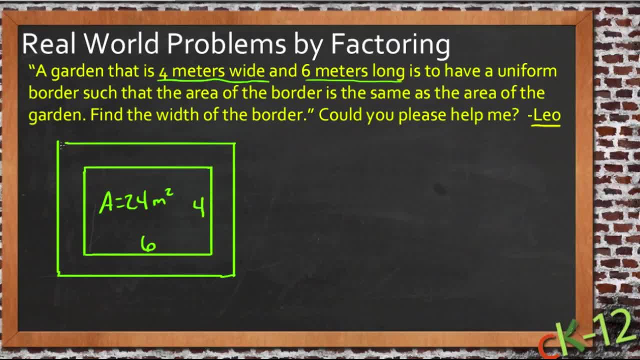 is uniform, then that extra width is going to be the same all the way around. Whatever this distance is- I'll change colors here real quick- whatever this distance from here to here is. 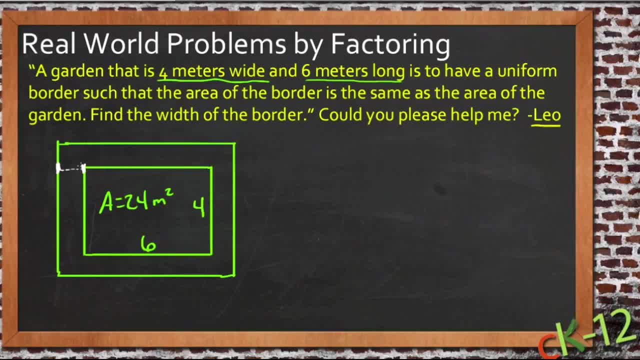 Will be the same all the way around. So that's what we're actually looking for: the width of that border. so that's where our variable needs to be. So let's call this distance here x- Now we know that the total—and we'll call this. 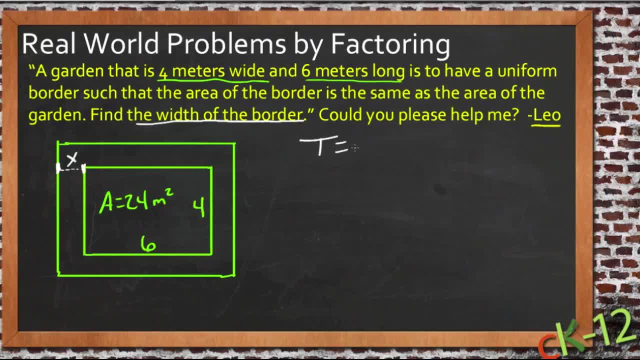 whole thing, the area of the complete thing. we'll call it t. t equals the total area. The total area then is going to be the long length here times the long reach length here, and if we want to find the width of the border, we need to find a. 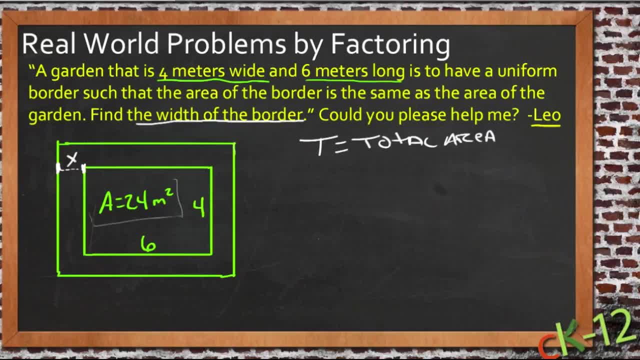 border to add on to this initial garden so that the total area of everything is twice as big as the initial area. so the total area, if it's going to be, if the area the border is going to be the same as the area of the garden, that total. 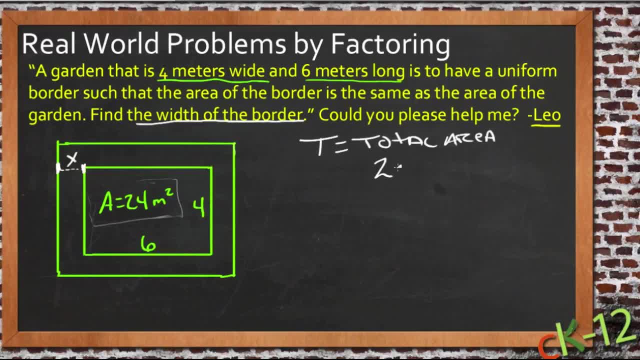 area is going to be 2 times the area of the garden, or 2 times 24 meters, which is, of course, 48 square meters. right? so then we just need to find a way to describe this total area. well, if the inside dimensions are 4 by 6, and what we're? 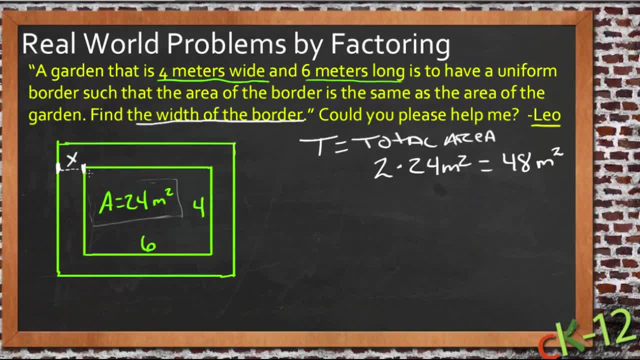 doing is adding this: this extra distance X to both sides, then this one here. this dimension here is going to be 4 plus 2x, because we're going to add 1 X distance here and 1 X distance here. and then this dimension across the bottom is going to be 6 plus 2x, because we're going to add 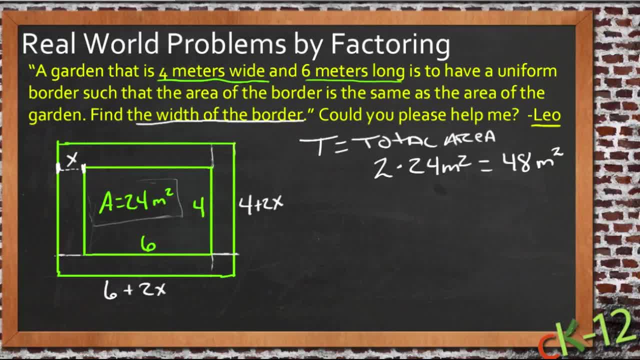 the X dimension here and the X dimension here. so this one, then, will have those, those two extra X's on the sides, and this one I have the two extra X's top and bottom. so 6 plus 2x is the new length and 4 plus 2x is the new width. so